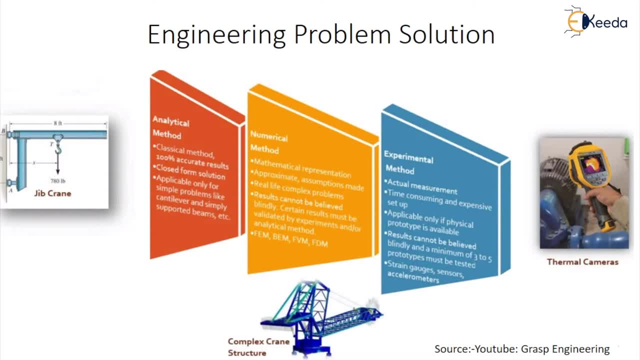 experiment or by analytical method. So FEM, BEM, FDM and FDM. these we will study in next slides. And experimental method is an experimental method where it is a time consuming and expensive setup. So we have to reduce in numerical method and applicable only for physical prototype which is available. 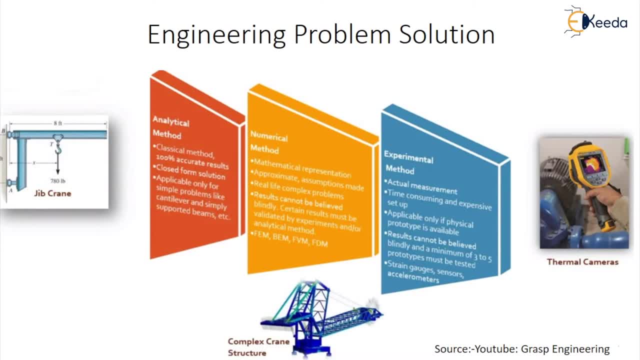 and results cannot be believed blindly here, and minimum 3 to 5 prototypes must be tested, and string-digit sensors- accelerometers, are required for doing any type of experimental analysis. For example, we are doing a crash test on 3 to 4 vehicles, So that is one of. 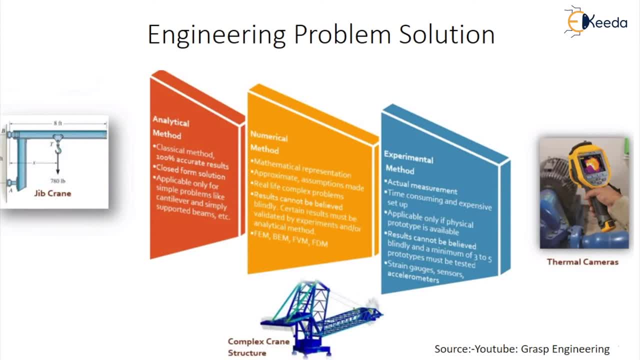 the part of experiment method. So numerical method, one of the three complex methods study shown in this, shown in the paper, while experimental process, onyl cameras are there and these tend for analytical method, We are having the results comparison with analytical methods. When you compare with analytical method, that means it is a very special case. So we are. 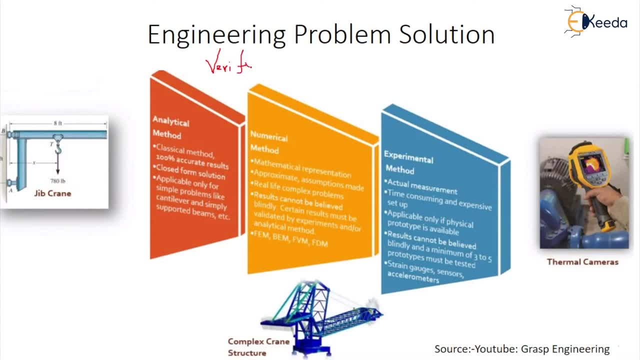 verifying the results with analytical method plate for analysis. we are being worried about lead high suivance. Then if that means comparison in between analytical and numerical, if comparison is in between numerical and experimental, that is nothing but validation. So remember this part is also very important- to understand what is validation and what 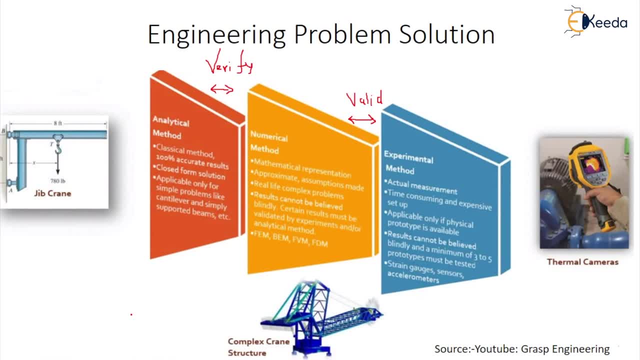 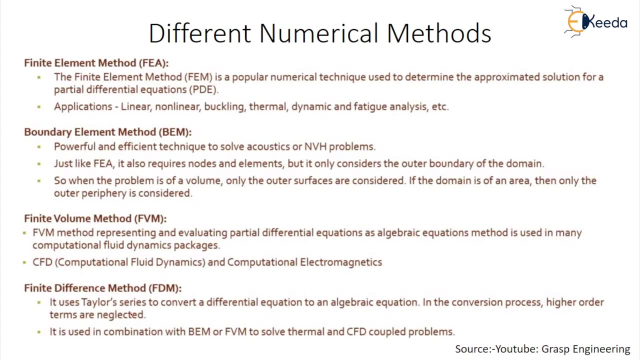 is the verification. Let's go to next slide. Different numerical method, that is FEM. So FEM is a numerical technique and it determines the approximate solution of partial differential equation. And applications are linear, non-linear, buckling, thermal, dynamic, static analysis. 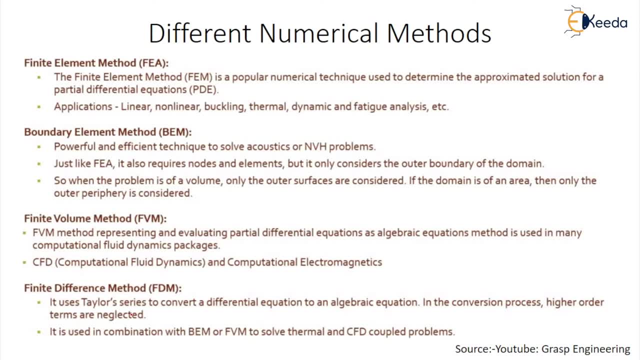 While boundary element method is a powerful essential for solving acoustic or NVH problem. NVH means noise, vibration and hardness problem. Just like FEM, it is also requires nodes, elements and but it is a fundamental method that is used to determine the process of evaluation of the surface. 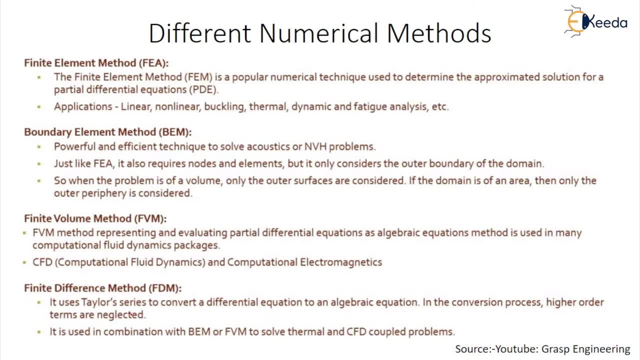 So, for example, if we consider only boundary, outer boundary domain, so it is a most of the surface or volume domain. So when we are taking a problem of volume, only outer surface is considered. It is a surface thickness. we are only considering the surface, not volume. 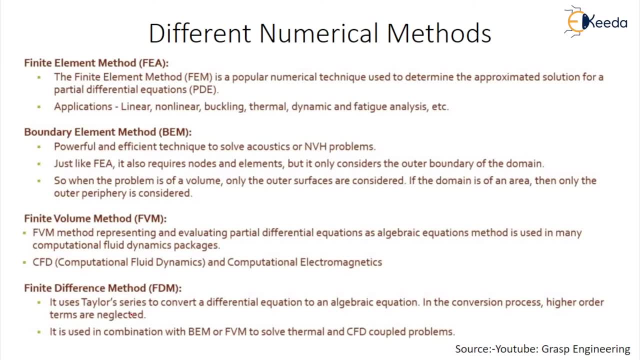 If the domain of an area, then only the outer periphery is considered, While finite volume method- the finite volume method is representing and evaluating the partial differential equation as a algebraic equation. So here it is. So it is an algebraic equation method in use of many computational fluid dynamics. 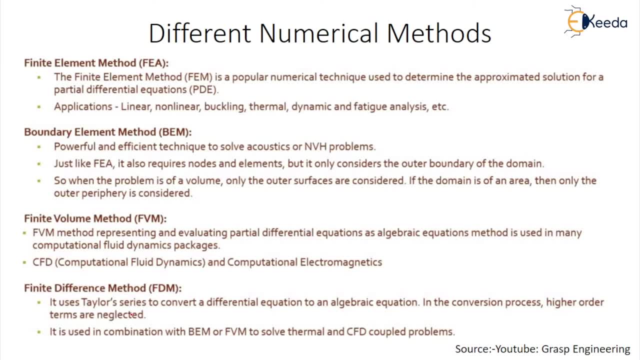 articles CFD and computational selection analysis, that is, comes under FDM, while FDM that is a Taylor series, convert differential equation to algebraic equation. in conversion process higher order terms are neglected and it is used in combination of boundary element method or finite volume method to solve the thermal and CFD coupled problem. 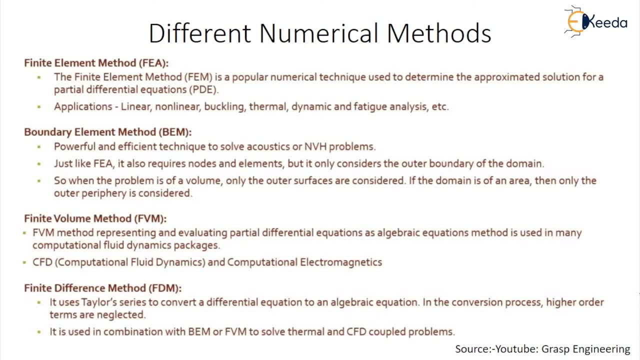 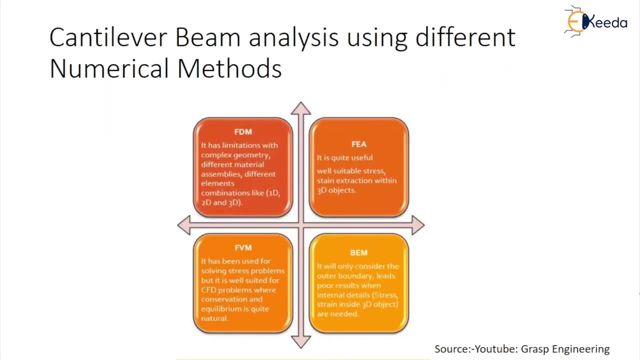 So it is always coupled with FEA and FVM problem or VEM problem. So if we are solving a cantilever beam analysis with all the analysis like FVM, FEA, FVM and VEM, then we get the answer, but FEA is the most suitable for cantilever beam instead. 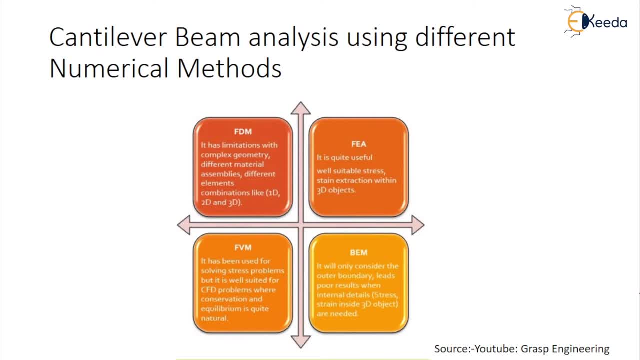 of FDM or FVM or VEM, How it is that FDM having a limitation with complex geometry, but for small geometries, different material assemblies and different element combination like 1D, 2D, 3D, So it is having a limitation, while FEA is a quite useful and suitable for any stress. 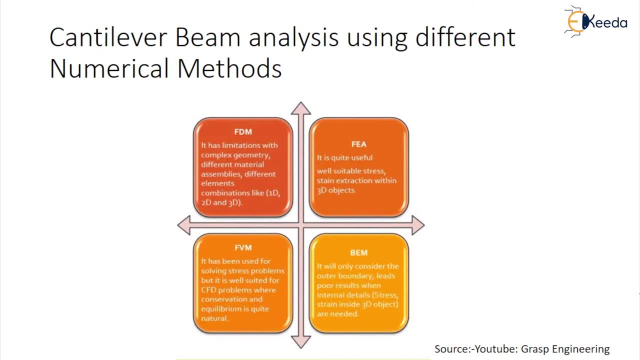 strain extraction within 3D object, while FVM is used for CFD problem with solving the stress problem, but it is more suitable for CFD and conversion and equilibrium of the beam. FVM is quite natural. Boundary element method is only considered as outer boundary. 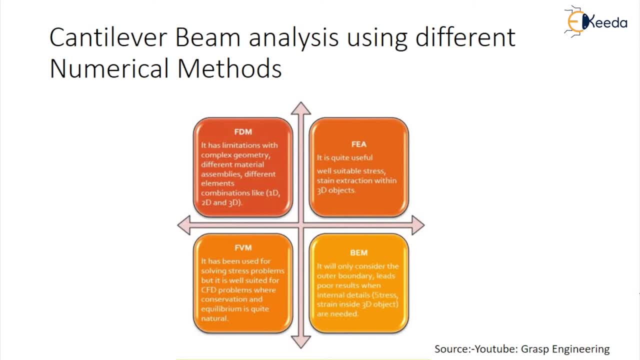 It is a surface with internal distress, direct phase strain and 3D objects are needed. So, according to the accuracy, according to the project time and according to the cost, these analysis are most important. You have to choose the analysis according whether we are going for upgrade or whether 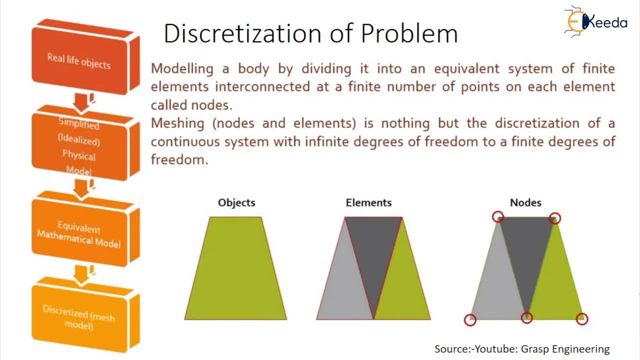 we are going for FVM. So discretization, That means real life problem. Real life problem is equivalent system for finite element which are interconnected with finite number of points on each element. that is called node. So this is the object. where, divided this object into triangular element with these: 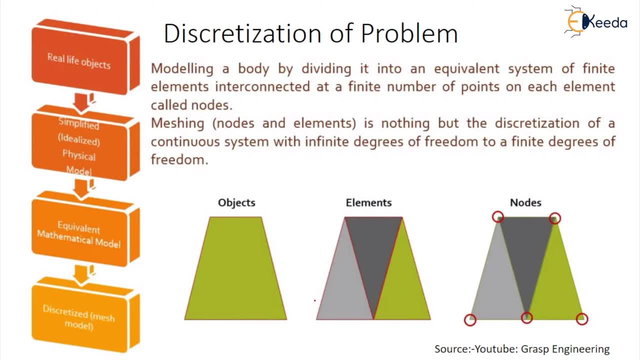 three triangles. So these are the three elements for this structure. and whatever the circles we have mentioned, those are nodes. So meshing is nothing but nodes and elements. So this is the structure of the measuring object: abolization of continuous distance with infinite degrees of freedom and finite degrees. 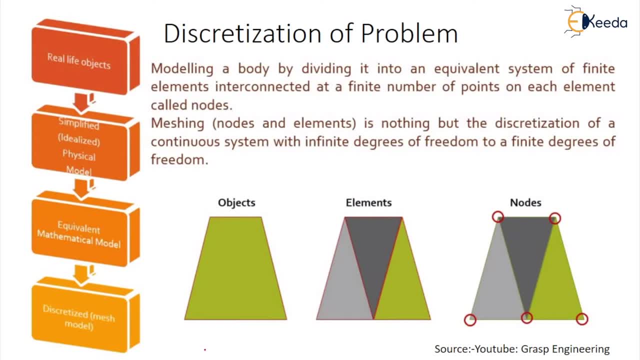 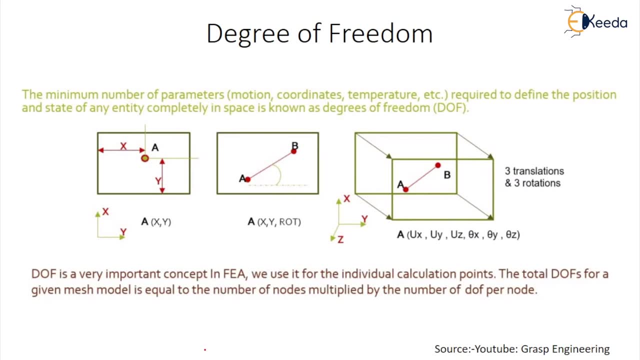 of freedom. So real life, object, simplified, idealizer, physical model, then convert it into mathematical model, then this is like mesh Degree of freedom, that is, minimum number of parameters, that is motion coordinate, temperature, etc. Those are required to define the position and the state of any entity completely in. 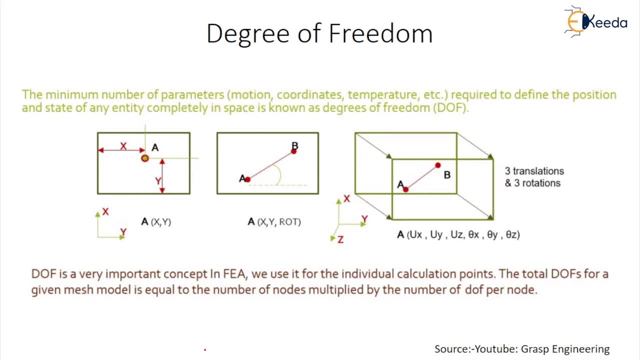 a state is known as degree of freedom, as degree of freedom. so in a particular space in this available, we have mentioned the x and y coordinate. okay, so it's having x and y is necessary, okay, while here x, y and rotation is given. so three degrees of freedom are given, okay for point two, while, uh, eight, any three. 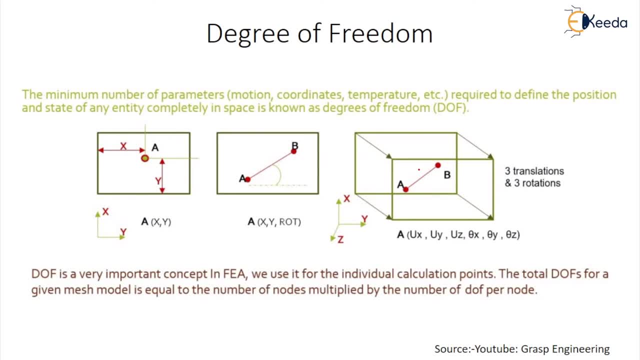 translation and rotation of a particular object, then it's having six degrees of freedom, that is x, y z translation, x y z rotation. okay, so dof is very important concept in fda and it is a individual calculation point. the total dos for a given mesh model is equal to number of nodes. 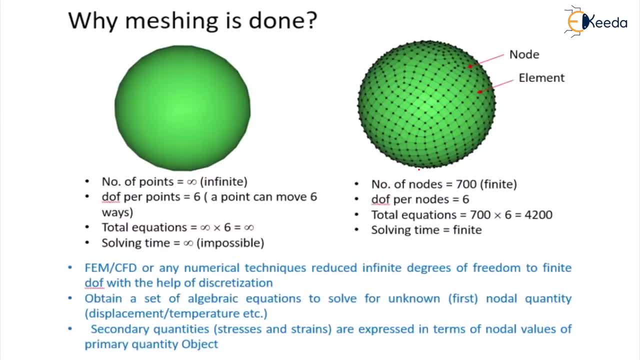 which is multiplied by number of dos per second. why meshing is done? the number of points, for example, we take a one ball and that time it is considered a number of pointer in final. okay, but we have to mesh, we have to discretize. that same number of nodes are 700. 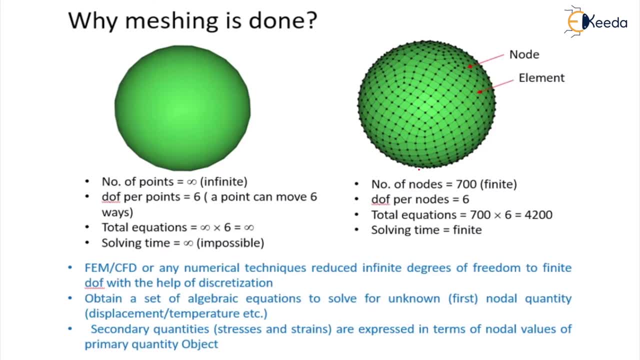 that is finite, that is we can easy to count. okay, then divide per uh points will be six. that is a point can move in six ways. here also a point can move in success. but there is 700, total equation infinite. following time is highly impossible, while total equations are finite. there is four thousand. 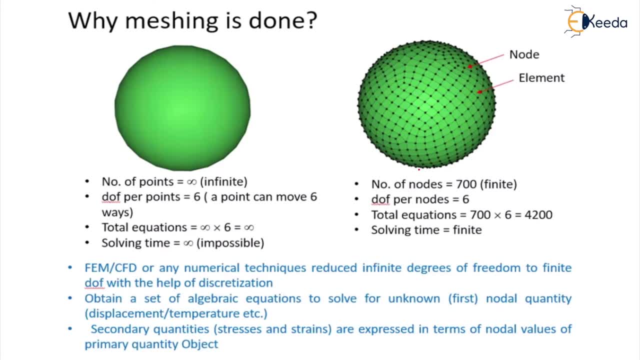 two hundred. following, time is final. so we can solve the particular problem, fem or pfd or any numerical technique reduced to infinite degrees of freedom, to finite degree of freedom, with the help of discretization, an opt-in set of algebraic equations to solve the unknown first, that is. 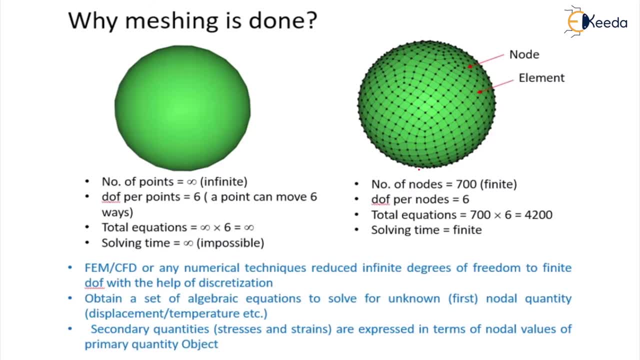 nodal quantity, that is displacement or temperature in thermal, and secondary quantities are straight strength. so there is a field variable that is actually working and there are secondary variables, that is space and strength. okay, those are secondary. from displacement we will get a strain and space, as everybody knows that space is proportional to 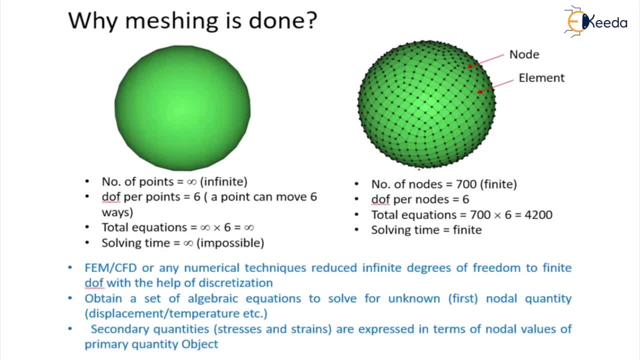 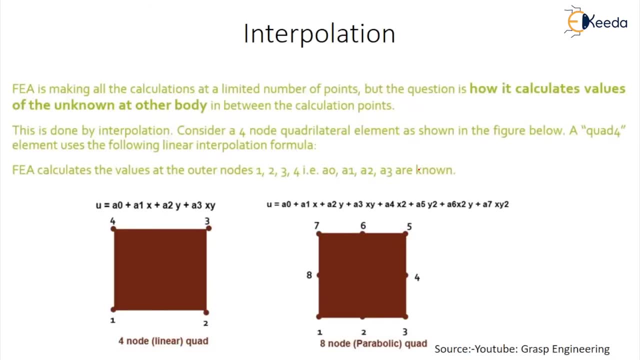 epsilon into and smallest, and space is equal to four square in the gradient. from that we can easily get the displacement or space and so okay. so interpolation, we are calculating this equation: u a naught, a 1 of x, a 2 of y or a 3 x y. 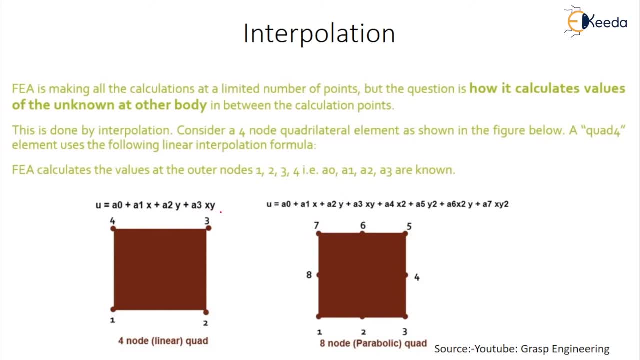 from the which, uh, from the pyramid. okay, so. so here there we are using a uh pyramid equation for- and these displacement equations are always at a node- 1, 2, 3 change. it calculates writing no zone, remember. so there is a four node, that is linear, quad, and 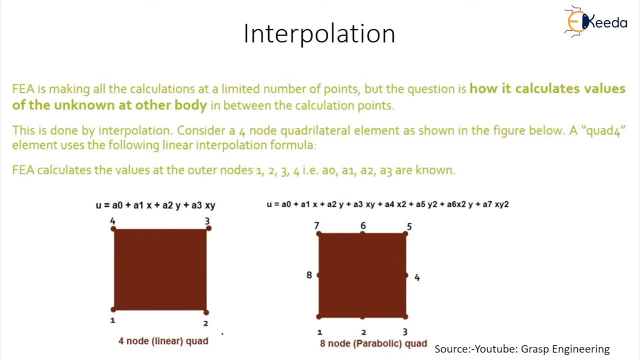 eight node, that is parabola. so uh, that is the p uh method where we are increasing number of modes. so there is a four node that is linear quad and eight node that is parabola. so that is a p method where we are increasing number of modes. 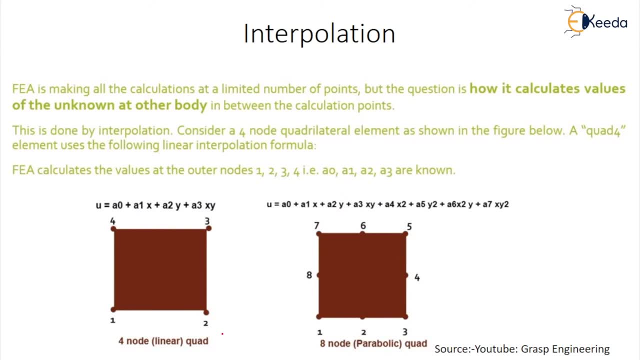 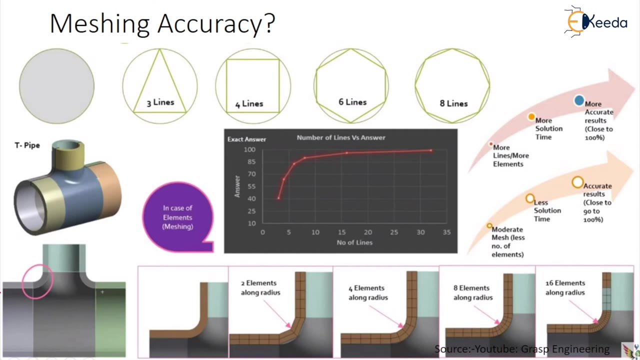 So it is a P element method. so quad 4 and quad 8. okay. so accordingly the result and time will be value. So machine accuracy is very important in every aspect. for example, we take a T pipe and we concentrate only on this particular cross section. that time we can, if we use two. 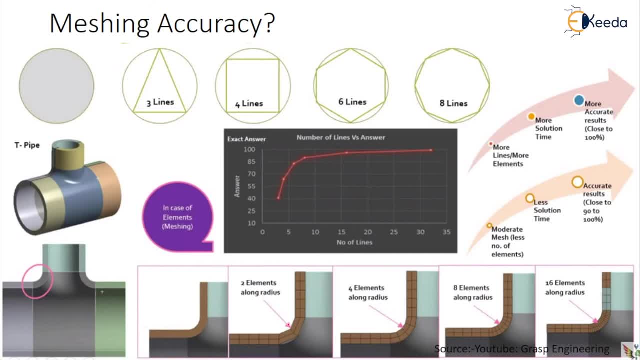 elements. it will not good for calculate and it will give not accurate or more to accurate result. while we go to 4 elements or 8 elements or 15 elements, it depends on that as a more lines or more elements we are using more solution time, it will take more accurate results that. 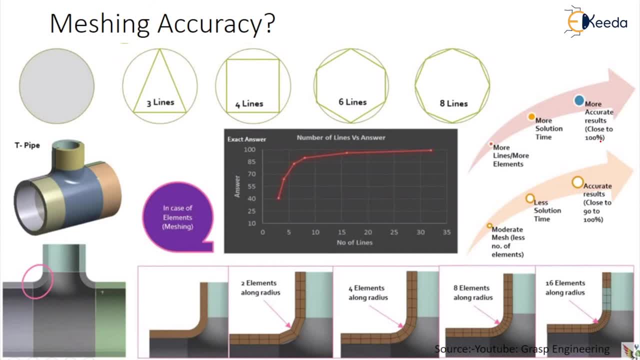 is close to 100 percent, but we use only moderate mesh. that is less than number of elements. for example, If here it is a very critical area, then either we can go for 8 elements or we can go for 4 elements. okay, so that will give the less solution time and accurate results. this closer. 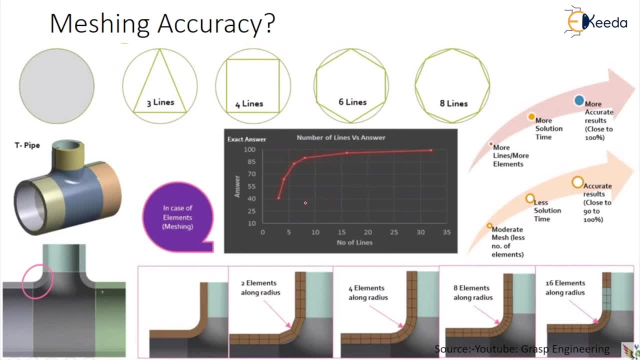 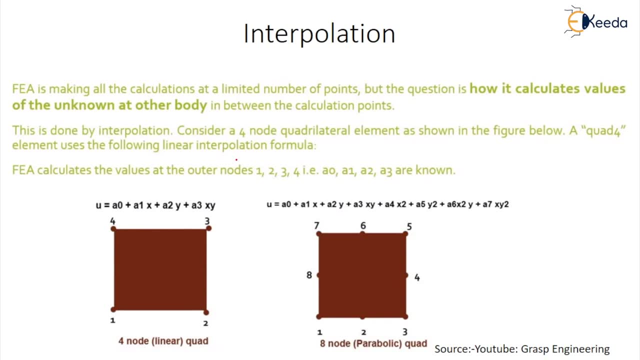 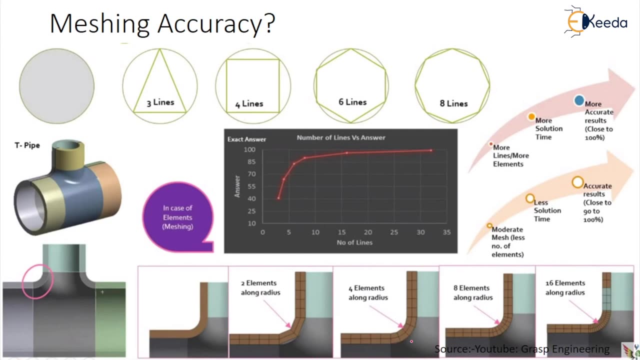 to 90 to 100 percent. this is the graph of number of lines versus answer. so previously we are increasing number of nodes in a particular element, so that is a P element method, while here we are increasing number of elements, so that is number of elements are increasing. 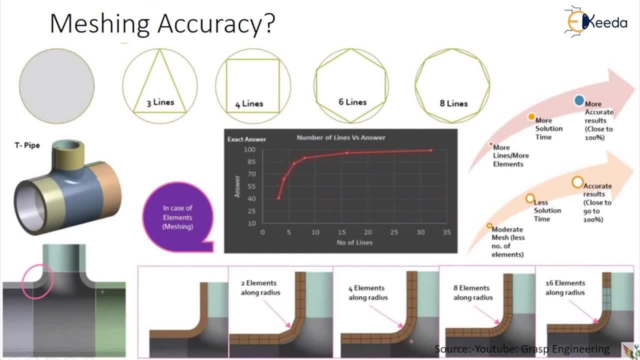 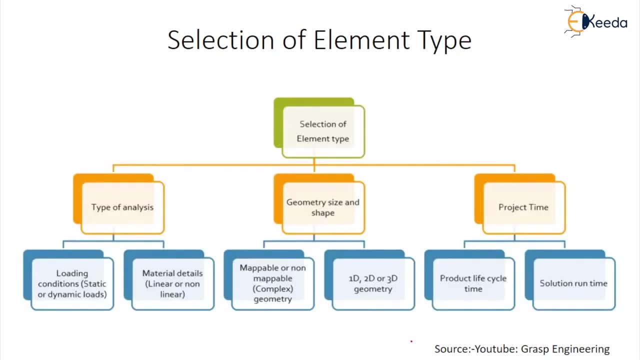 that means number of lines are increasing. then it will give to the exact answer. so it is a H element, okay, so remember this one. then selection of element type depends on type of analysis: loading condition, material condition, and then geometry and size shape. we have a mappable, non-mappable. 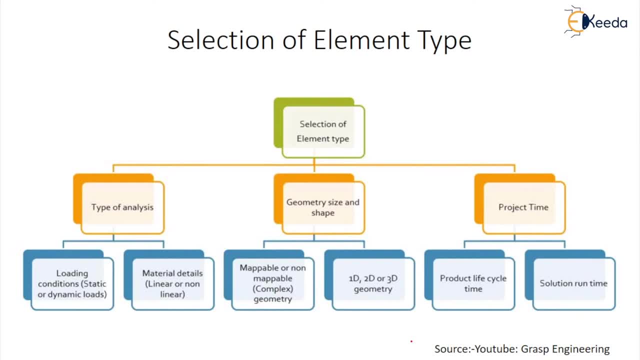 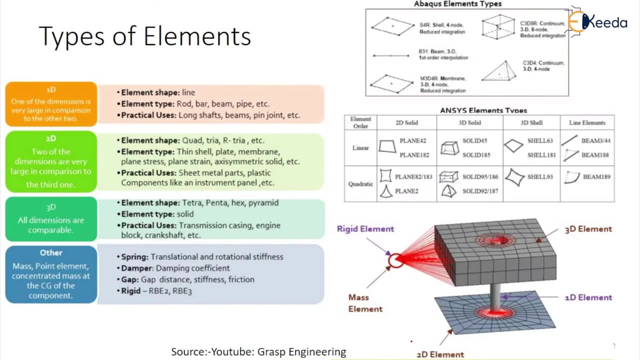 complex geometry or 1D, 2D or 3D, shape and project time. it is product life cycle time and solution value. type of elements are for 1D: line elements are there, that is, rod b, bar, beam, pipe, etc. you practically use this long, sharp beams in joint etc. while 2D elements are quadra, tria, r, tria etc. 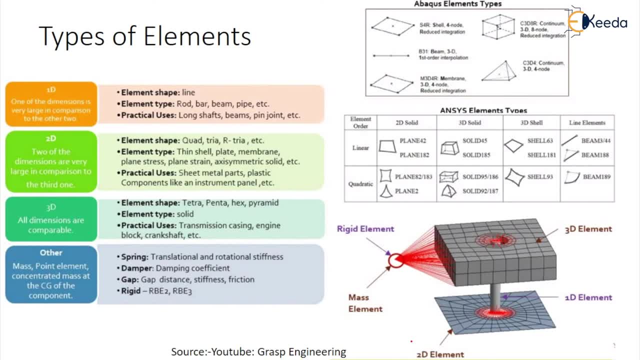 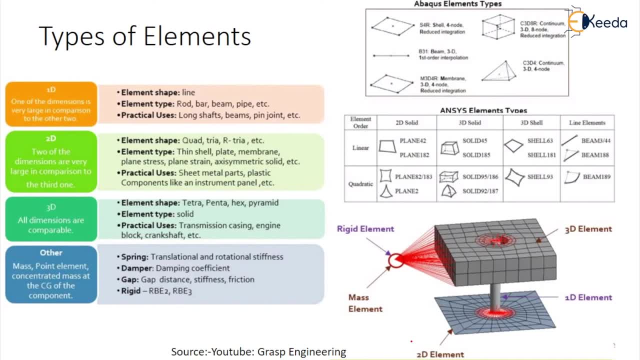 So tria means a regular shape of triangle or mostly equilateral triangle, While quad is our square. okay, so thin shell, plate, membrane, plane, stress, plane, strain, axisymmetric, solid, etc. practical uses are sheet metal parts, plastic components like instrumental panel for 3D dimensions, tetra, penta, x pyramid. these are used where solid element type and the 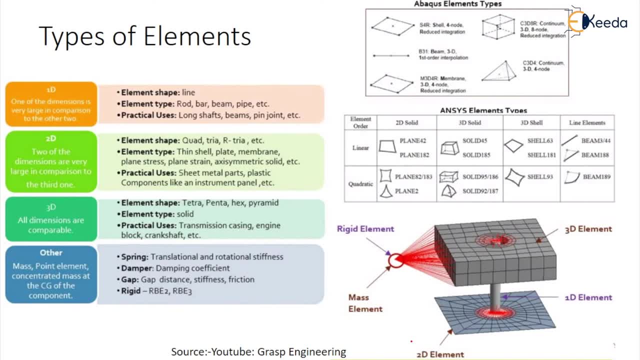 transmission casing, engine block, crankshaft, etc. we are used and there are some other elements. types are translation, rotational stiffness, damping coefficient, gap distance, then stiffness friction, that is rbe2, rbe3.. So here there are different abacus element types, or linear quadratic types are shown in this figure. 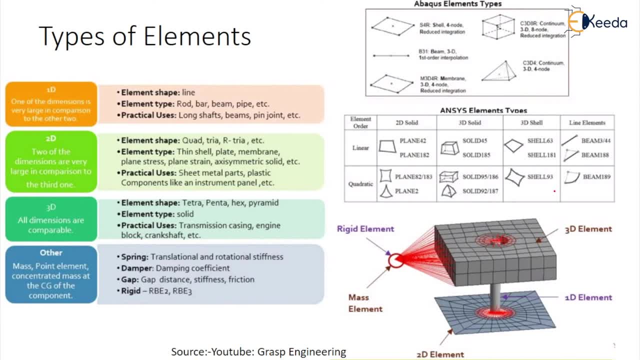 where you will get a. this is a hexa. okay, this is a tetra. so this type of equation we are getting on every type of element type or every type of 1D, 2D or 3D and mass element. okay, So rigid element is shown in this figure, that is, a mass element as 3D elements in the hexa form. okay, 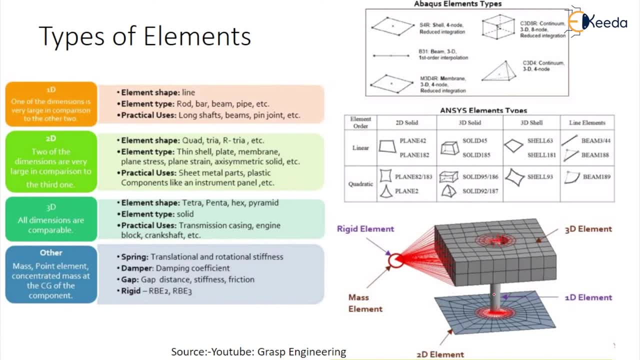 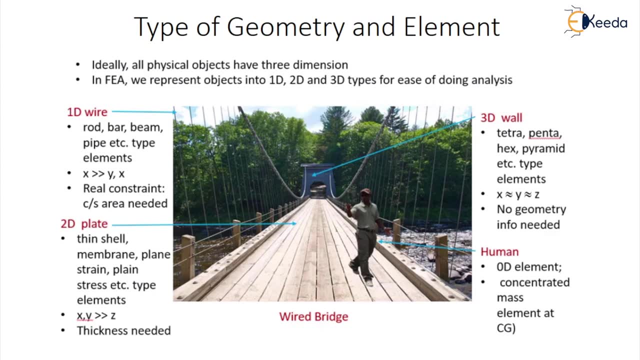 So here it is a 1D element, so middle, that is 1D element and this is surface, where it is a 2D element. okay then, type of geometry and element: again those things are mentioned in a practical form that a wired bridge is there. So where wires are 1D wire, where x is very, very greater than y and x. 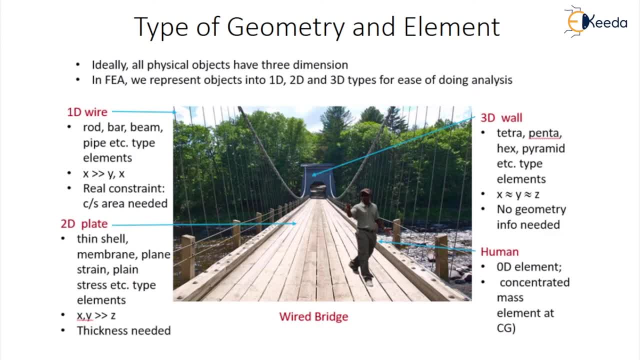 So where wires are: 1D wire, where x is very, very greater than y and x, While 2D plate is our path of the bridge. so that is a membrane plate in plain strain condition where x, y is more greater than z and thickness is measured, while 3D wall, that is tetra. 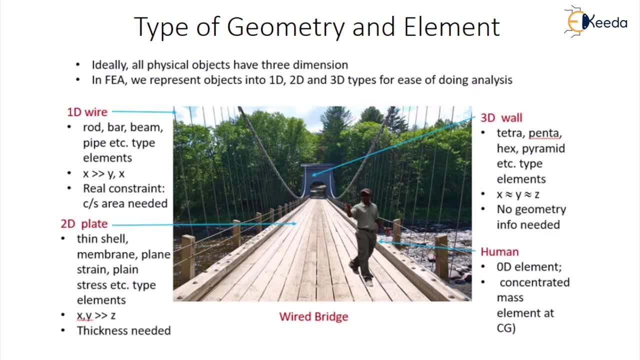 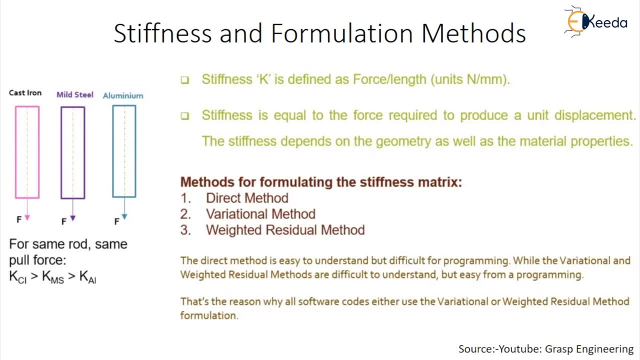 penta, hexa and pyramid is considered, while human is a concentrated mass element at e. Stiffness and formulation method, where stiffness case define force per unit- length, that is, unit- while stiffness is equal to required or producer unit. displacement and the stiffness depends on the 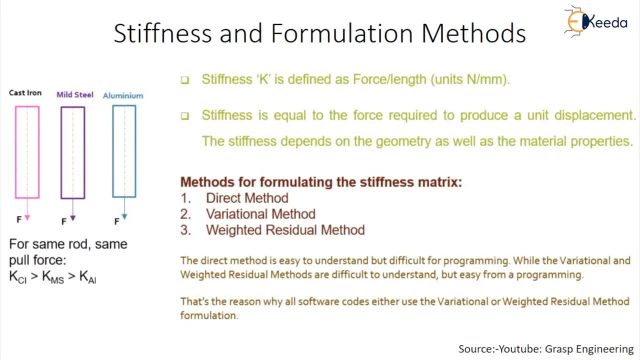 geometry as well as material purpose. So methods of formulating stiffness matrix such as direct variational vector distribution: okay. for same rod, same full force, k of ti is greater than k of ms is greater than k of al. the direct method is easy to understand the difficulties for programming: 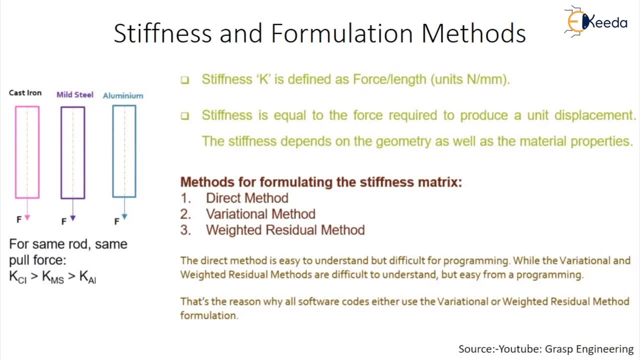 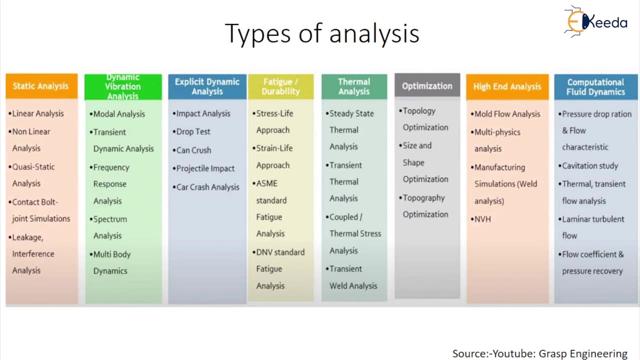 while variational and weighted distribution is difficult to understand but easy for programming, And that is a part of programming that is behind the software types of analysis: static dynamic, vibration analysis, explicit dynamic analysis, fatigue, durability, thermal analysis, optimization, high-end analysis, computational freedom. so static analysis having linear, non-linear 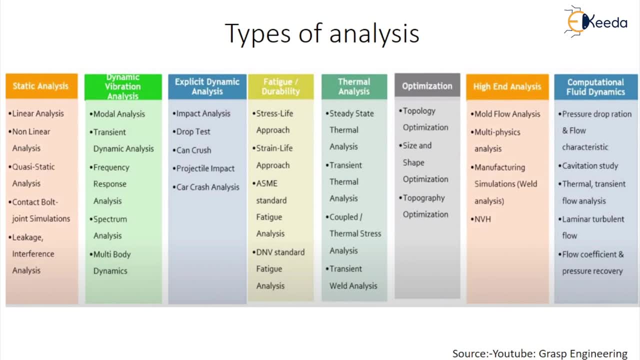 quasi-static for a short period of time. then contact ball joint simulation. or it's having a leakage interference analysis. it's having the buckling analysis is also considered in a static while dynamic vibration model analysis, transient dynamic frequency response, spectrum analysis, multi-body dynamics. so explicit dynamic analysis having impact analysis of a car. then drop test of. 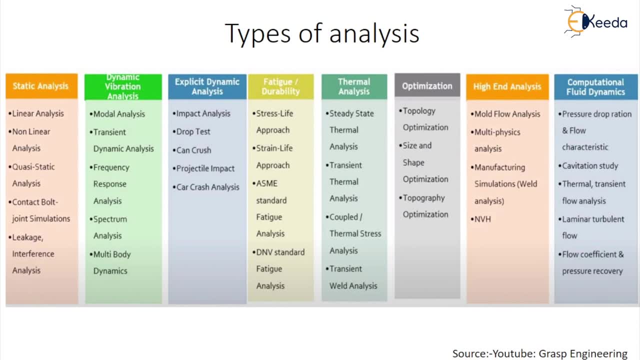 a unique ball on the car bonnet, then car can crash. crash analysis, projectile impact, car crash analysis, purchase durability is a mean. so this life approach, same life approach asm, is standard fatigue analysis or dlb standard fatigue analysis, thermal analysis having steady state transient 決신. 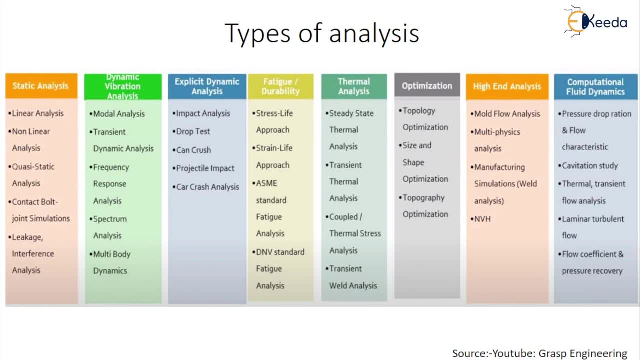 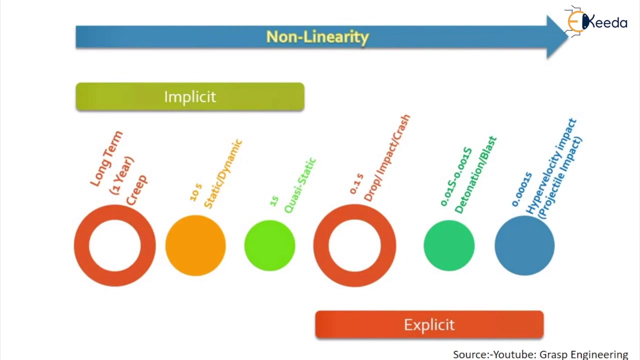 alleine, having pressure drop ration and flow characteristic, while cavitation study, then thermal and transient flow analysis in laminar turbulent flow analysis and flow flow from coefficient and pressure recovery analysis, Then non-linearity for implicit and explicit. implicit for very shortest period of time. 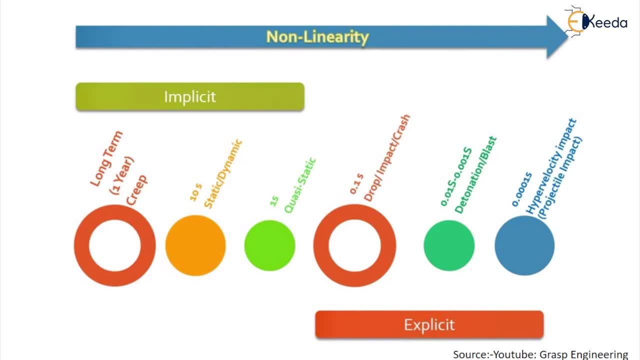 that is acting on a particular object to long term or 1 year. 3 conditions, where static or dynamic condition for 10 seconds and 1 second for process static, While explicit analysis, that is, drop, impact and crash, so these are considered under very less shortest period of time, while implicit analysis, taken for very last time domain, while 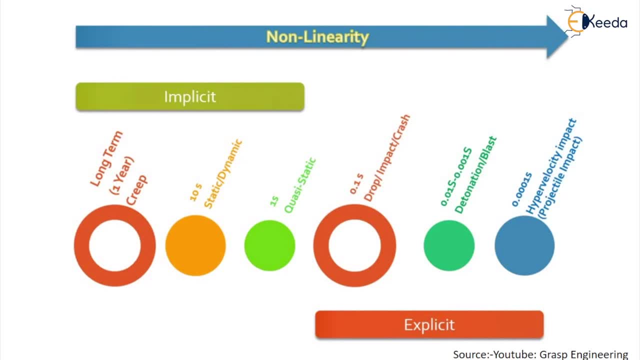 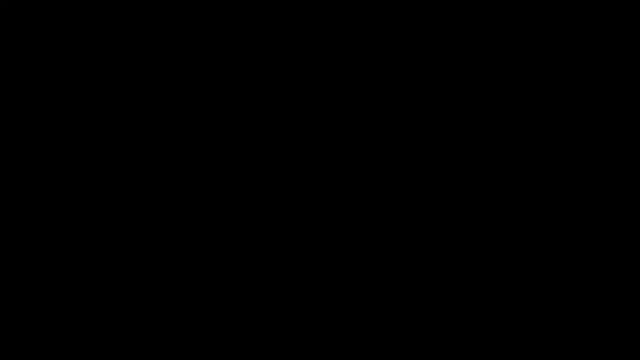 explicit for shortest or very quick. that is detonation blast, Then Motion, projectile motion or motion of a bullet. so those are considered under explicit analysis. Thank you so much. hope you understand very well. Thank you.